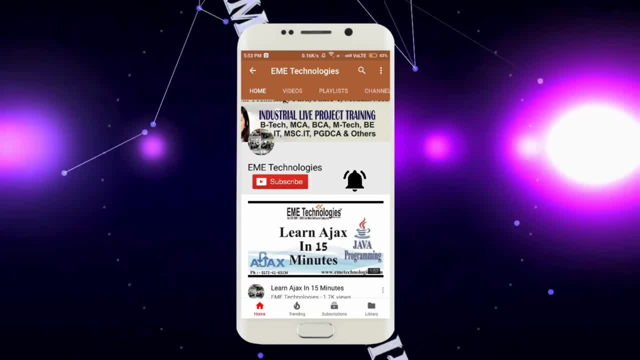 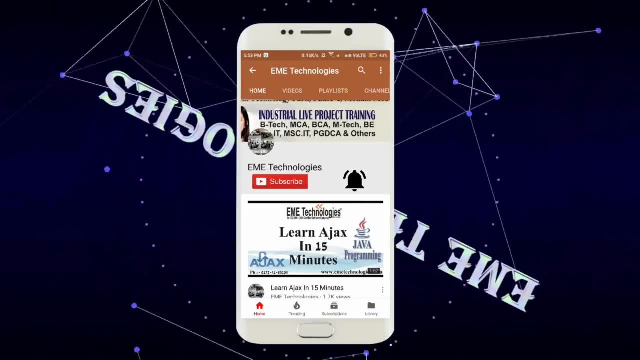 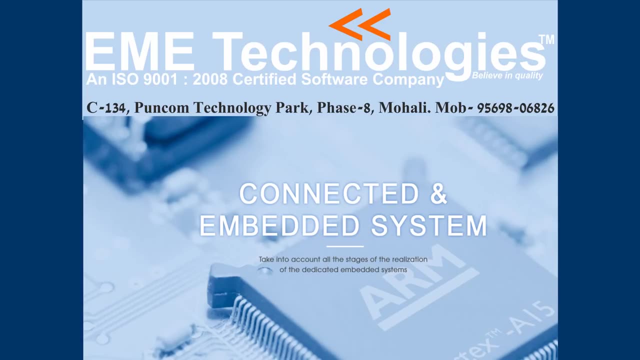 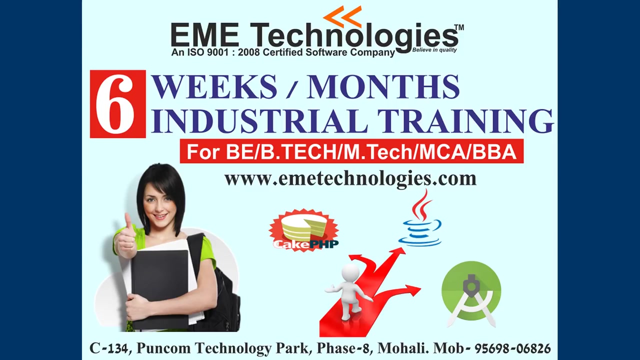 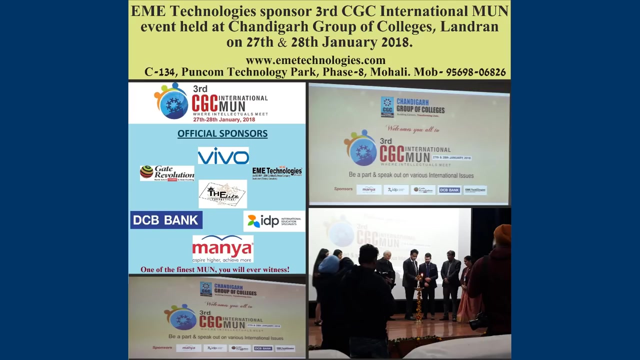 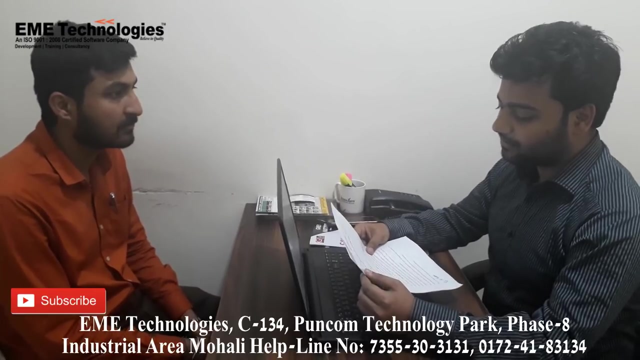 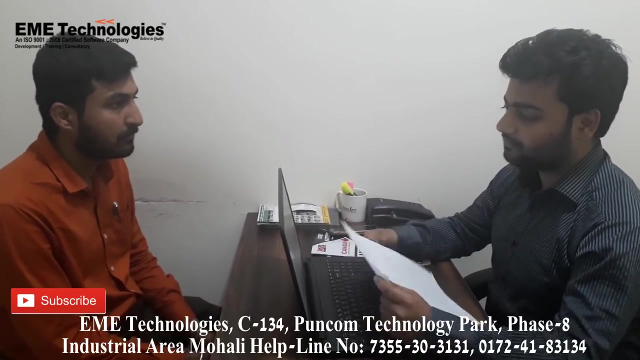 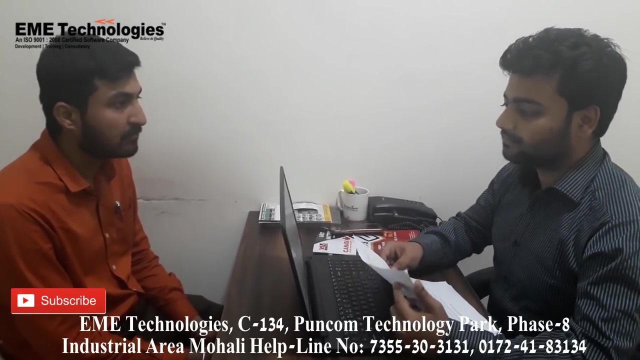 Hello everyone. I am from EME Technologies. Welcome to this channel. Please subscribe our channel and press the bell icon for latest updates. Good morning, sir. Good morning So, Mr Akash. tell me something about yourself. Sir, my name is Akash Singh, I belong to Amritsar and my father is a job in Punjab State Power Corporation Limited And my mother is housewife. I am pursuing my BTech from Amritsar DA College. 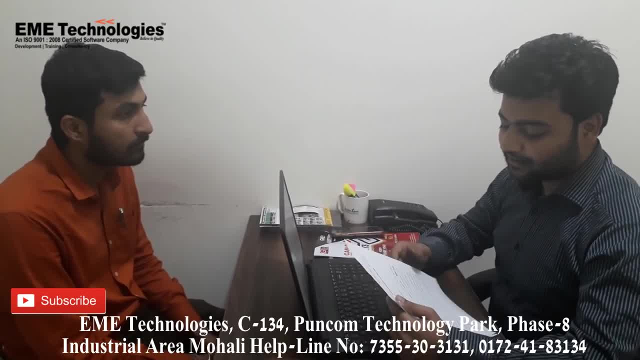 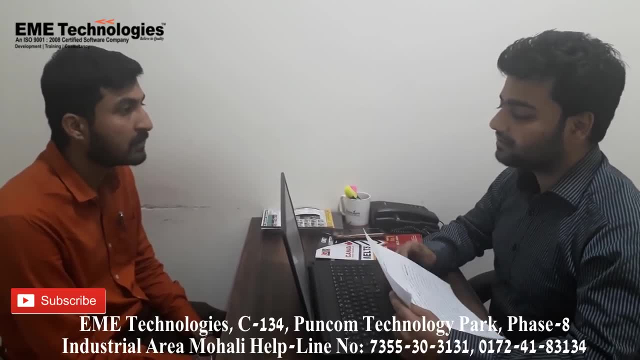 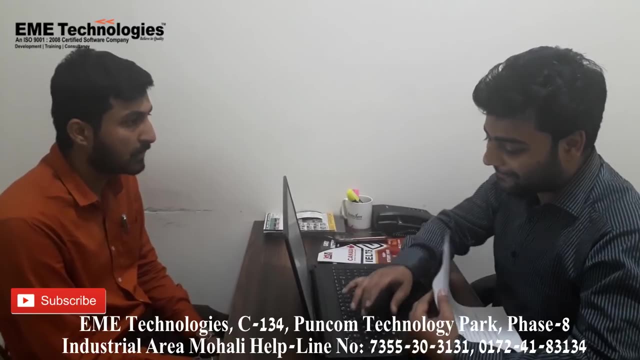 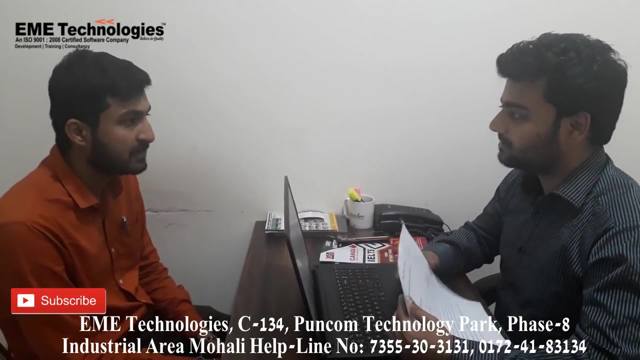 Okay. So what is your name? My name is Amritsar DA College. I belong to Amritsar DA College. I am pursuing my BTech from Amritsar DA College. You have done your BTech in Electrical and Electronics Engineering. Yes, sir. Do you know about resistances? Yes, What is the working of resistance, Sir? resistance: drop the voltage- Yes. So do you know about the color coating of resistance? Yes, sir. Okay, What will be the color coating of 10 kilo ohm resistance? 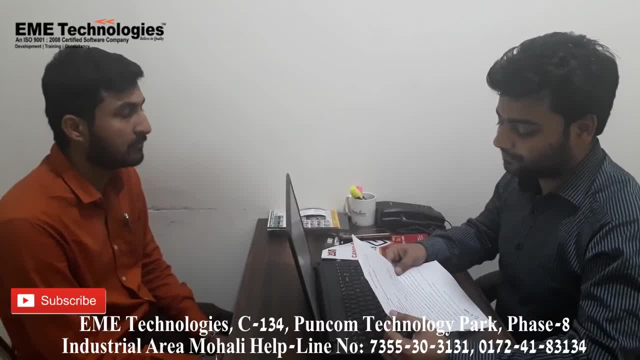 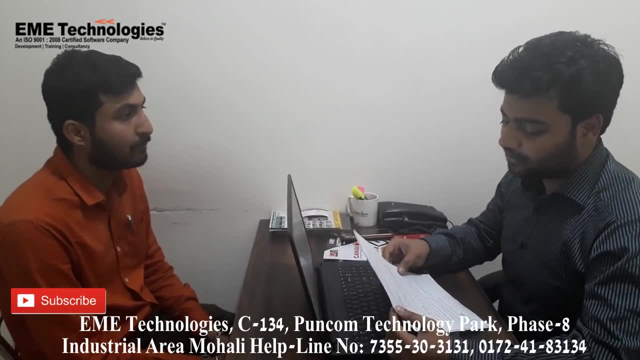 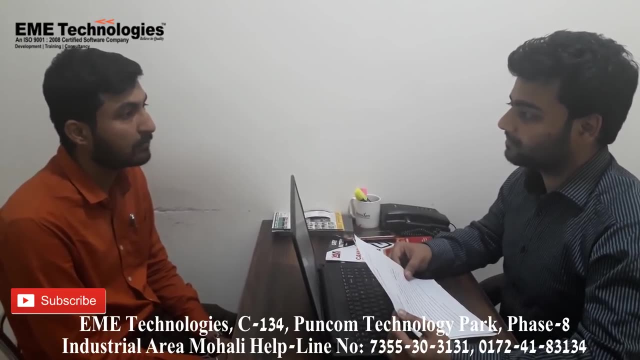 Sir, 10 kilo. ohm, Sir, 10 kilo. ohm, Sir, brown, black brown, black brown, Brown, black brown. it's wrong. 10 kilo, ohm, Sir, 10 kilo. ohm, Sir, Brown, black brown. No, it's wrong, Yes, sir. 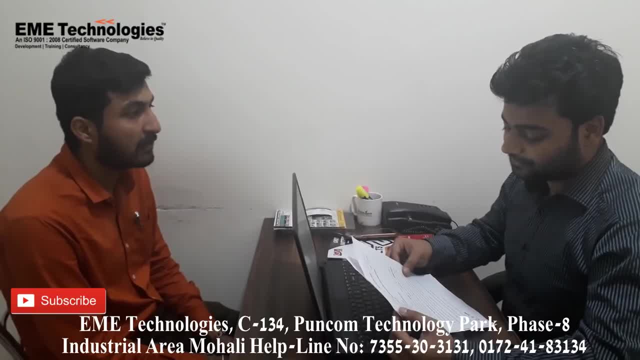 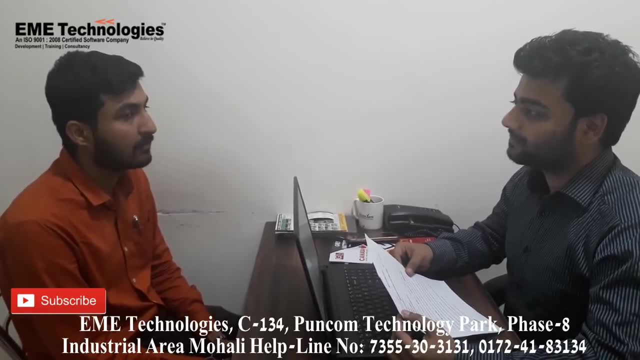 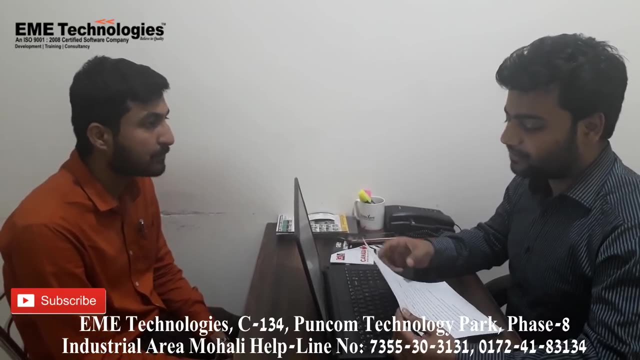 What about 1 kilo ohm, Sir brown, black red? Yes, this is right. So what about 10 kilo ohms, Sir Brown, black brown, black orange? yes, that's right. yes, okay, so as smd surface mount devices are already used in. 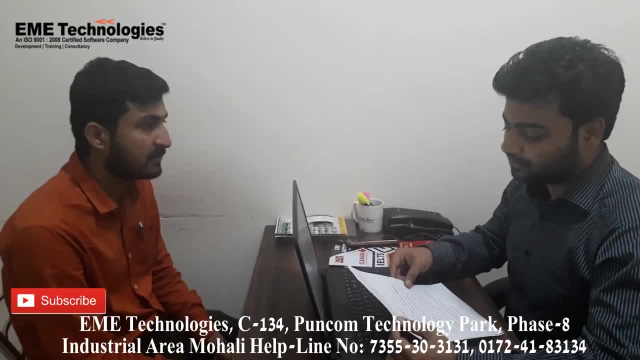 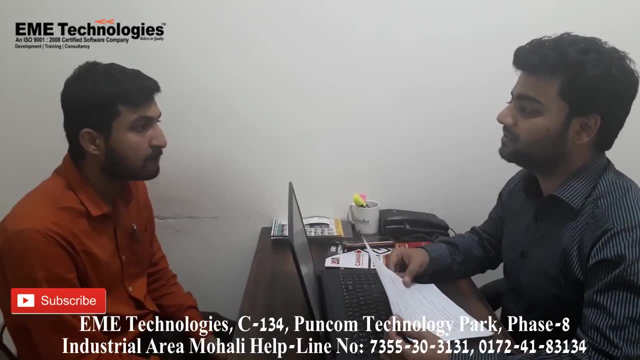 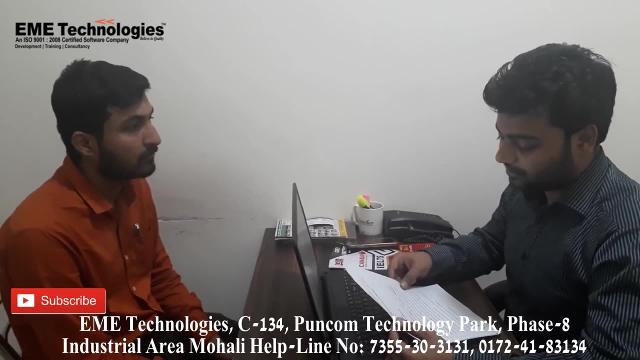 every project or every electrical appliance. so you should know about the assembly resistances also. so what will be the numerical value? if the numeric value is 331, what will be the value of resistance? so it's very, it it's very. three thirty, ohm, three thousand, yeah, that's right. and uh, two to one. 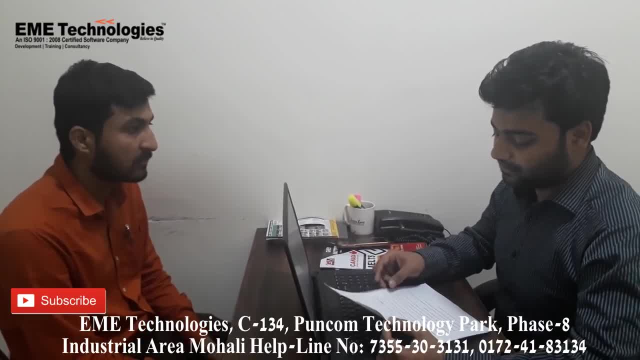 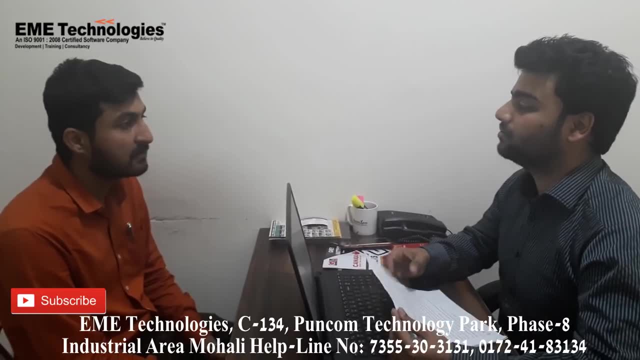 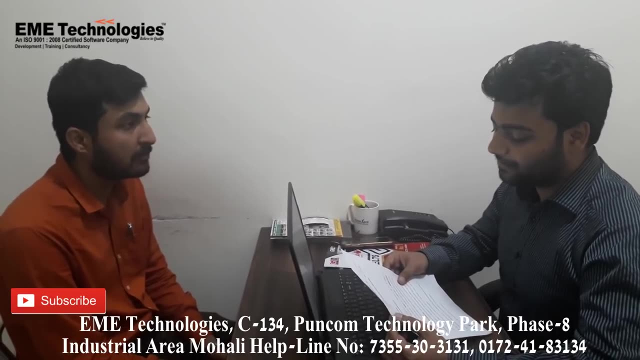 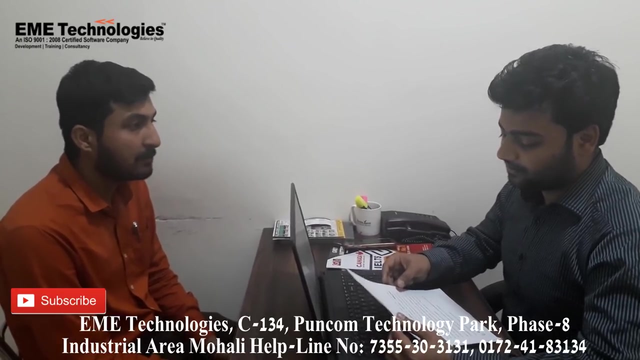 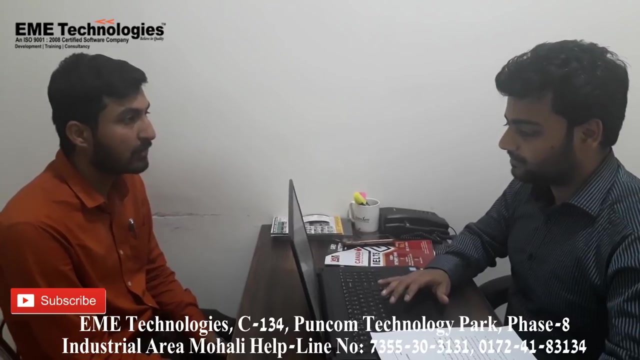 so it's very two, twenty ohm. yes, that's right. so, uh, these are the resistances. after that, what about transistors, sir? sir, two types of transistors. name them is the basic difference between them, sir. in p and p, we give the, we give some some amount of, some amount of ground to, to run the. 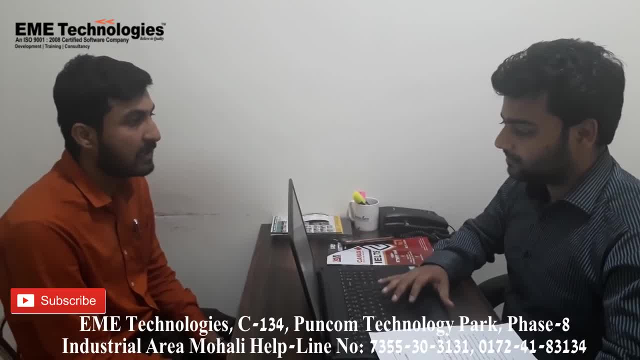 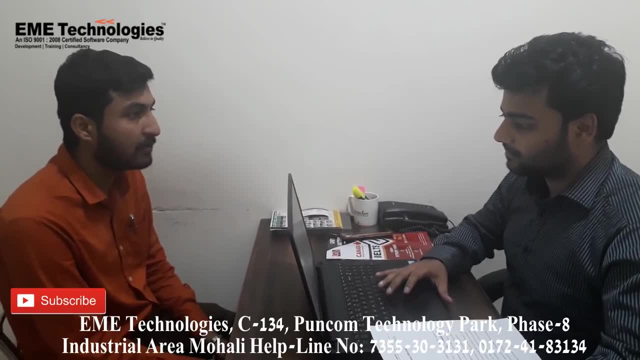 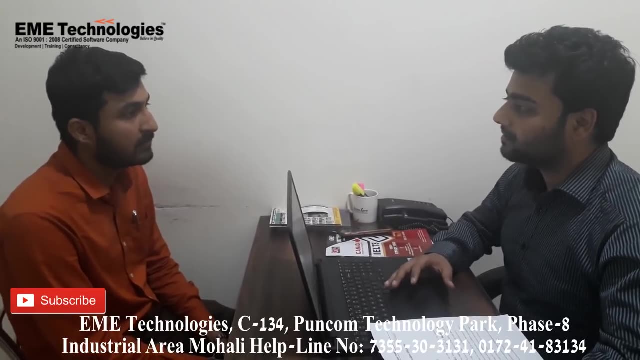 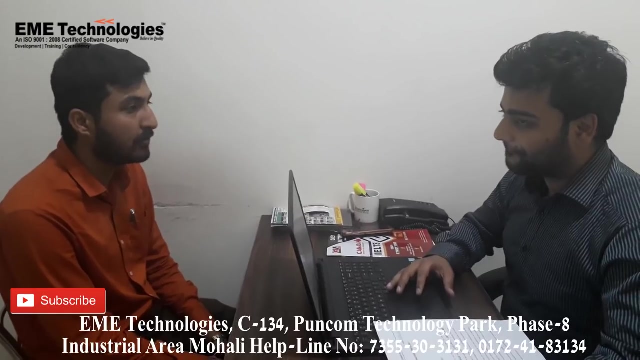 to to run the draw, to run the transistor and in p and p a week in at in npn we give some voltage to to base, to to run the transistor and in pnp certainly p and p we give. then p and p we, we, we give the ground to run the, to run the trans. 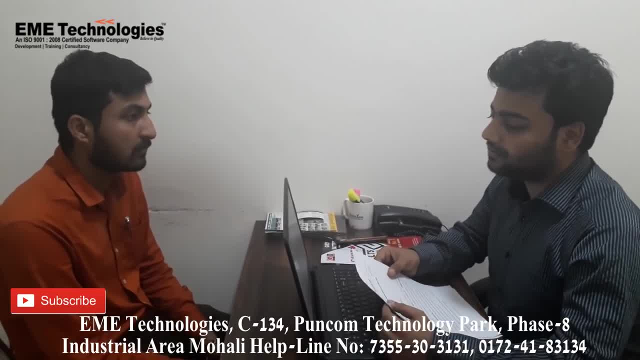 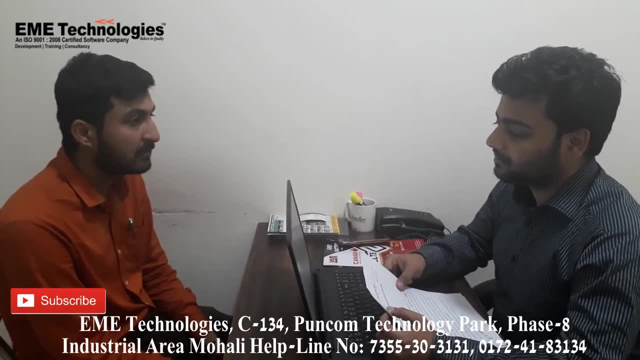 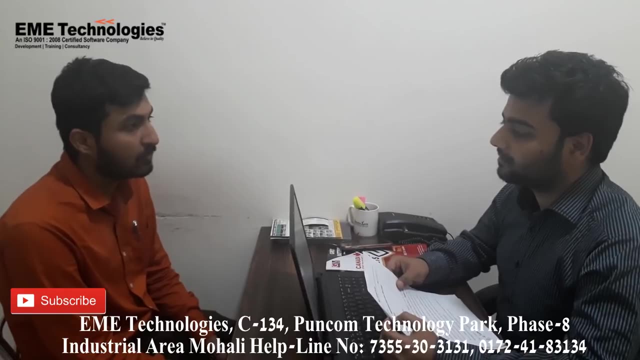 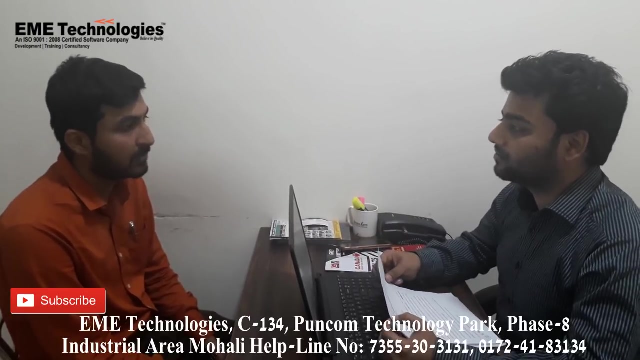 standard. okay, uh, what? for what purpose? we use diodes, now the injection diodes. so we we use that, we make the, we make the rectifier bridges to convert ac to dc- yes, and also we use the current in in uniform traction, So we can use it for production purpose also. 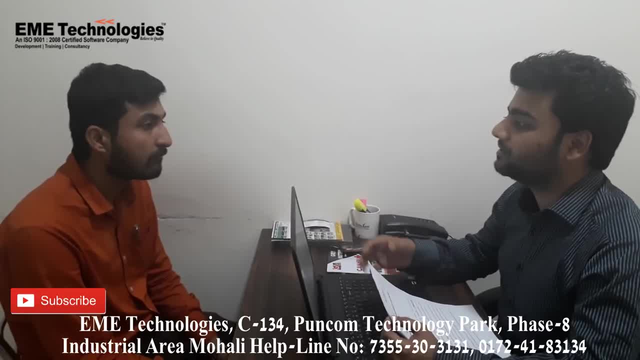 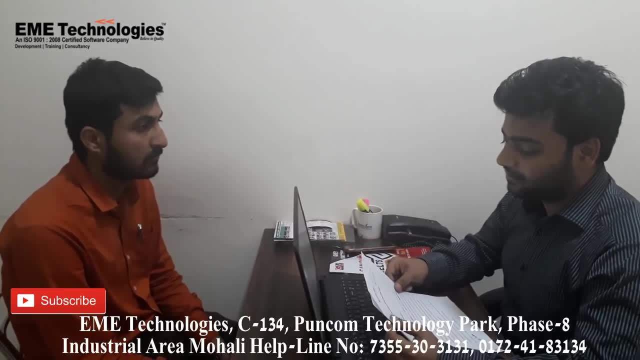 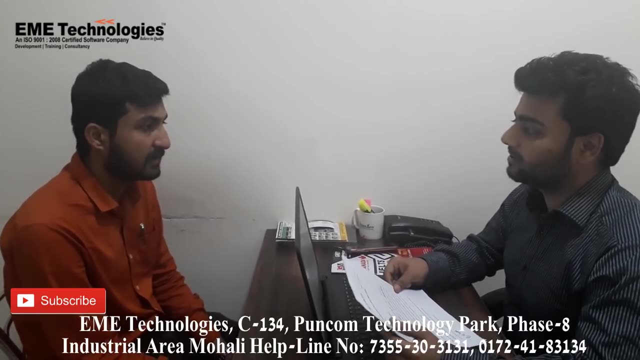 Yes, sir, As these diodes always conducting forward bias, Forward bias, It will not conducting reverse bias, Reverse bias. yes, So after that, you have mentioned that you have done a project on 8051 based home automation. Yes, sir, 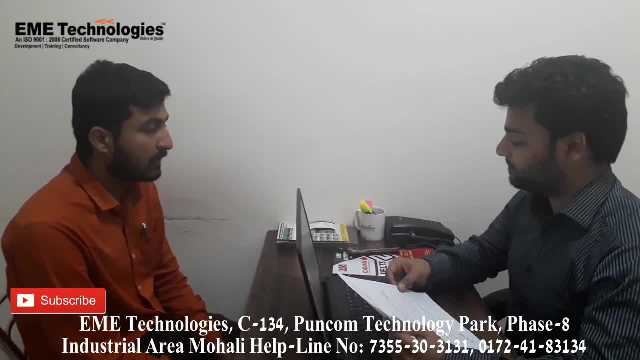 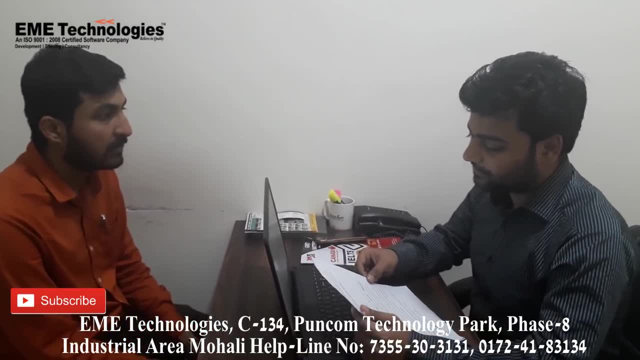 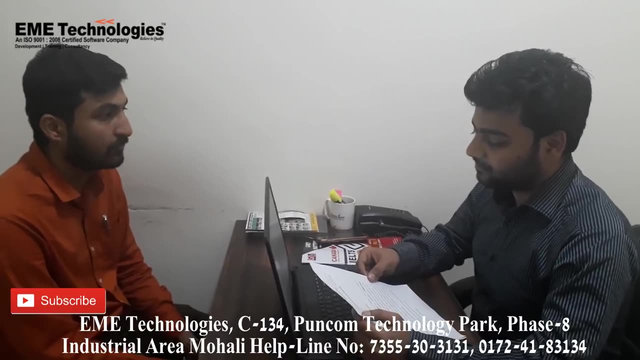 So what components did you use in this project, Sir? I have used 8051 micrometer with transistor, relay and capacitor. Okay, And some power Power supply section. Yes, sir, So can you make a power supply section on this stage? 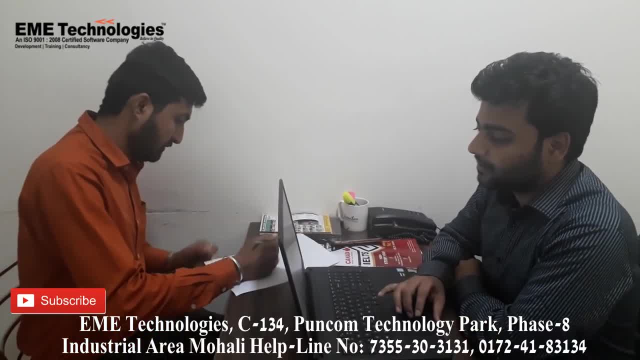 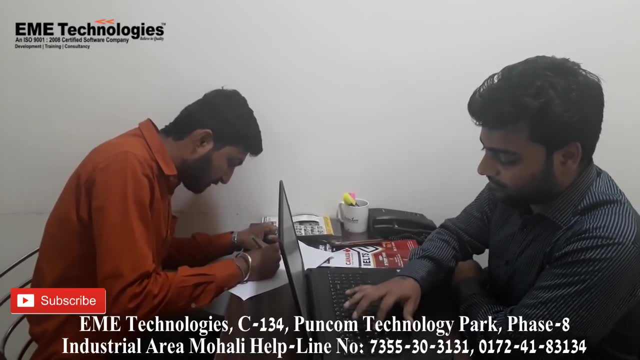 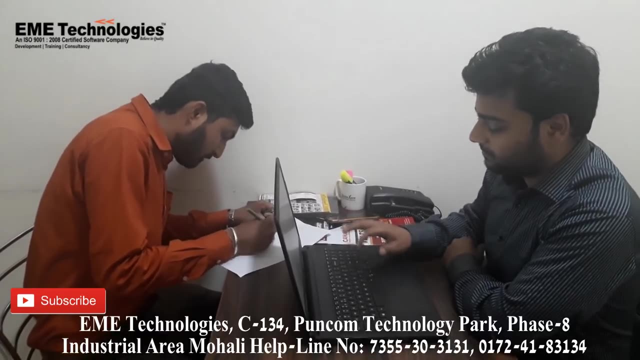 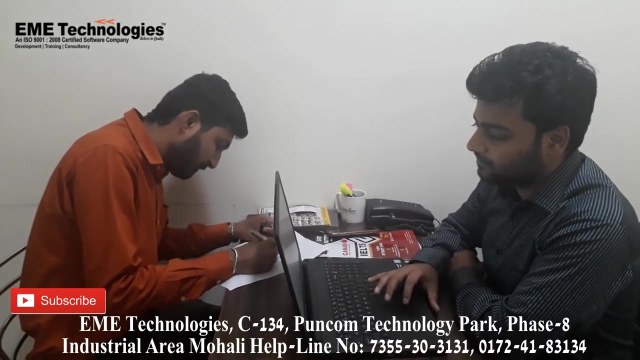 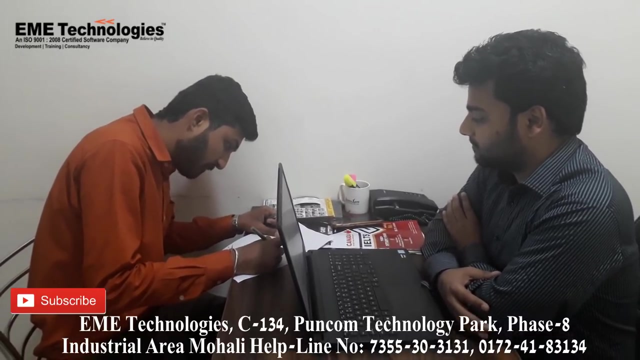 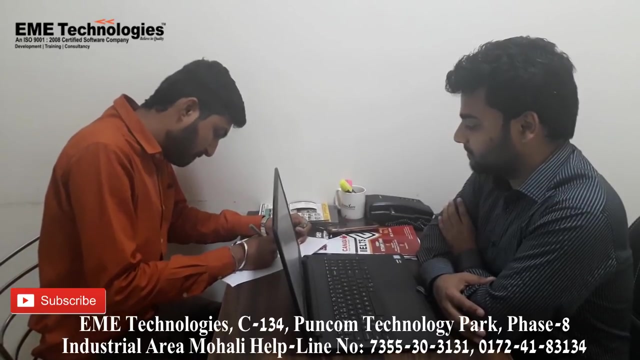 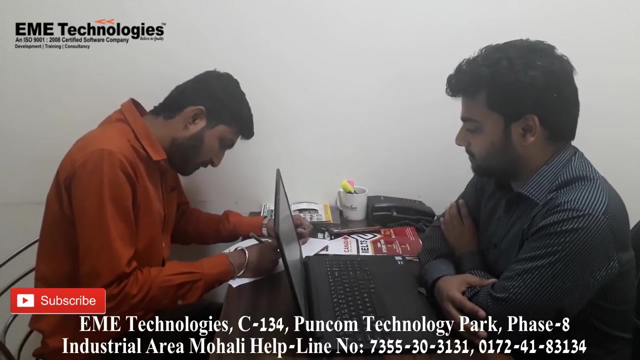 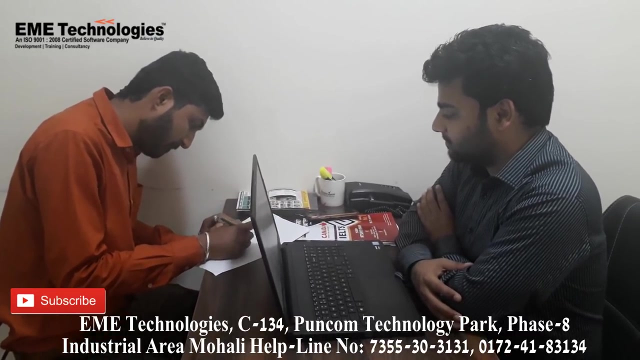 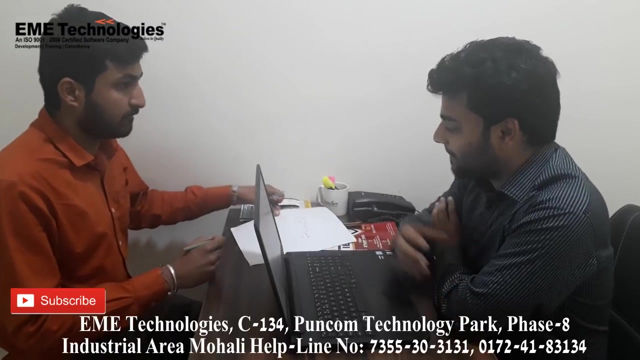 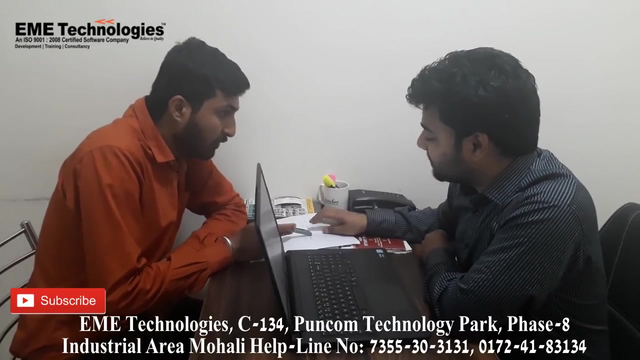 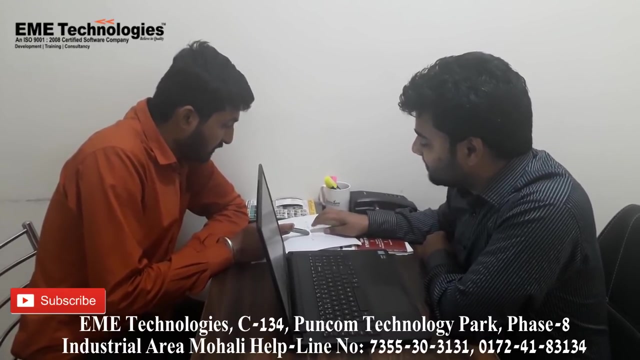 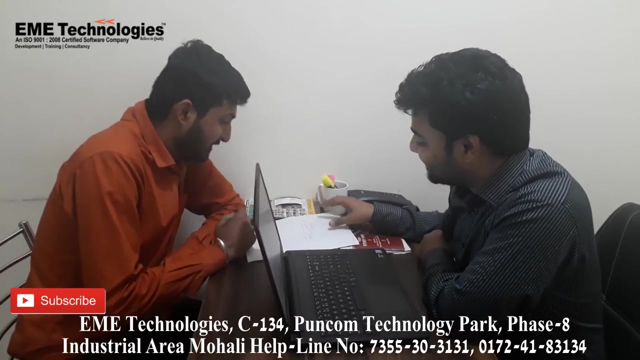 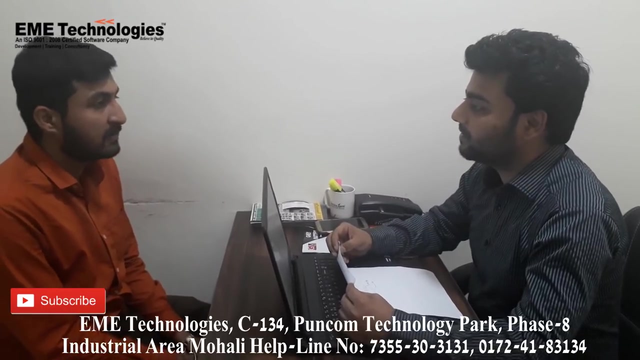 Yes, And also the DC power station. The DC power station and it should be connected, Connected, And then it is connected. There you go. what is this part? this is a micrometer, this is transistor, and what is this part? this is a capacitor. so about 8051 micrometer. how many ports are there in 8051 micrometer, sir? 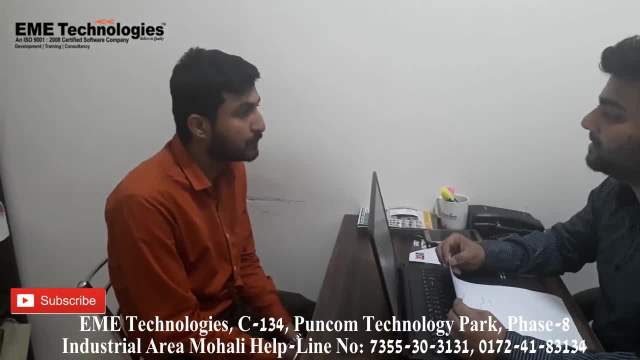 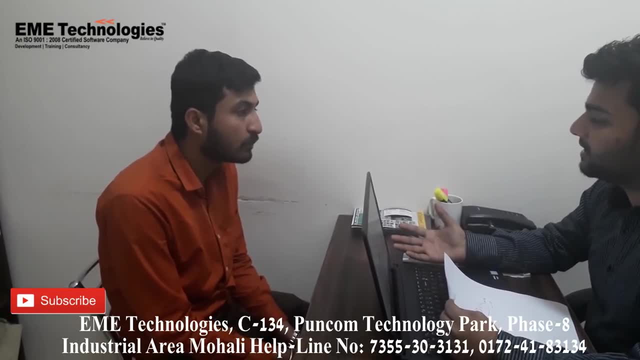 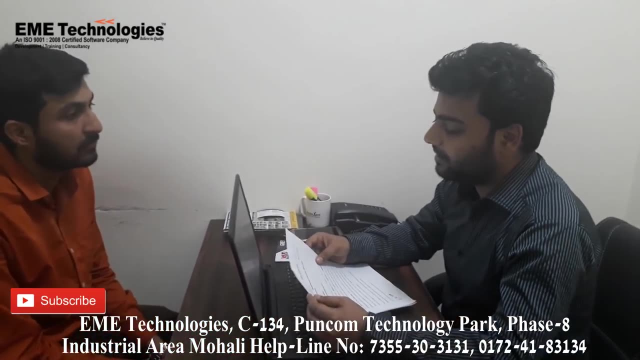 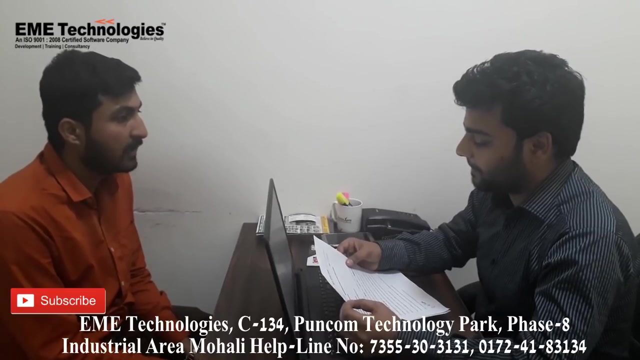 4 ports and how many pins, sir? 40 pin, and can you differentiate in special function pins and general purpose pins, sir? sir, 32 is general purpose pin and theta is special purpose pin. how do you name them, sir? PCC, ground reset, clock, external memory. ok, and external memory. 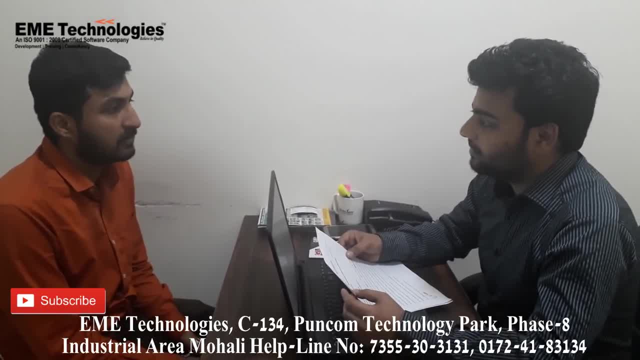 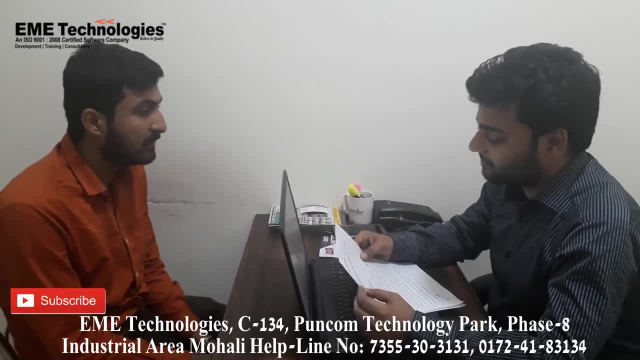 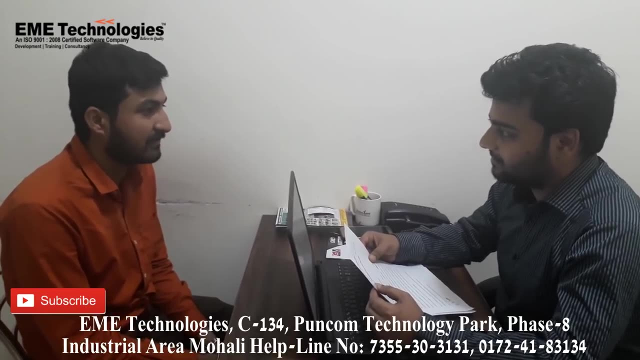 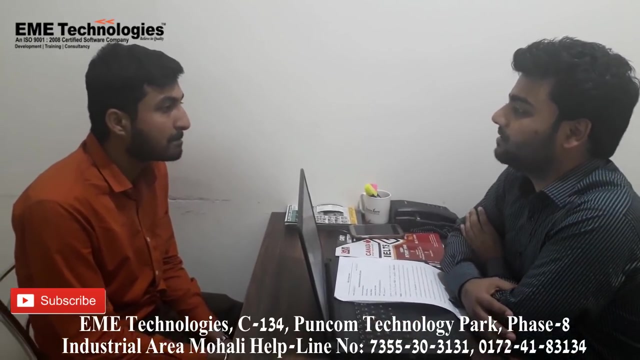 PCC and clock clock 8. you name them. these are 6, 2 left, 2 left, PCC, ground reset clock and 14 pin 쏭s, sir, reset, reset. you already name them. reset pin. wait, no problem, how much frequency of clock we used.